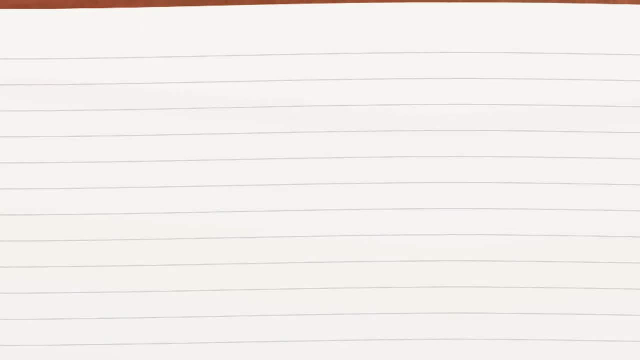 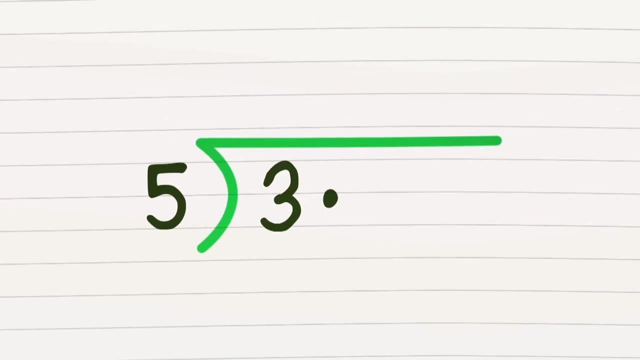 decimal. getting to the point isn't really too technical. So let's start by giving three fifths a try. It's like saying three that's divided by five. Now, five don't really go into three, but if you tried thirty it'd be easier to see. And now that we know, 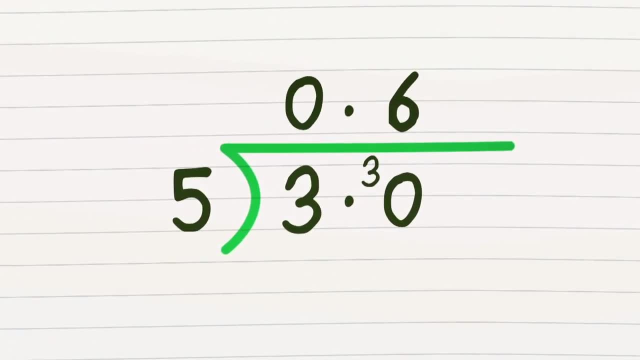 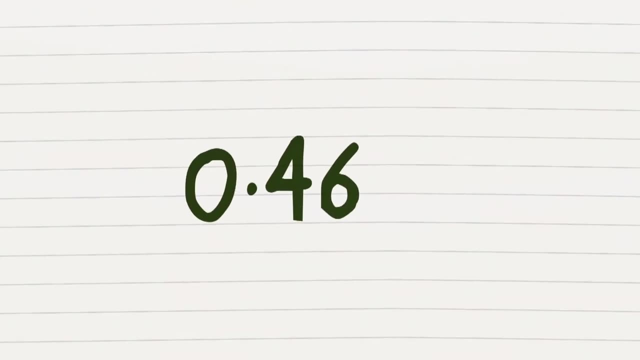 the main number that fits. divide it again to get 0.6.. To get from a decimal over to percentage, multiply it up by one hundred to get it. So if you start with a 0.46, move the numbers two to the left forty-six From decimal to percentage. it was multiplied, but 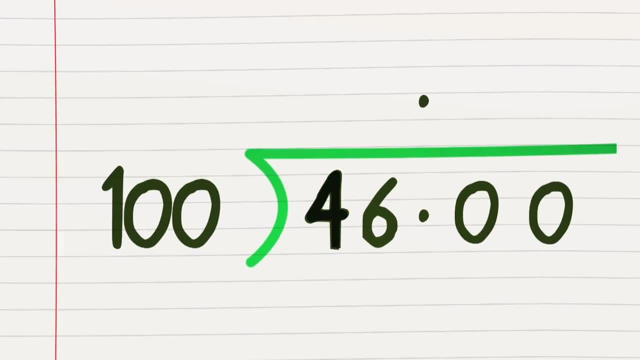 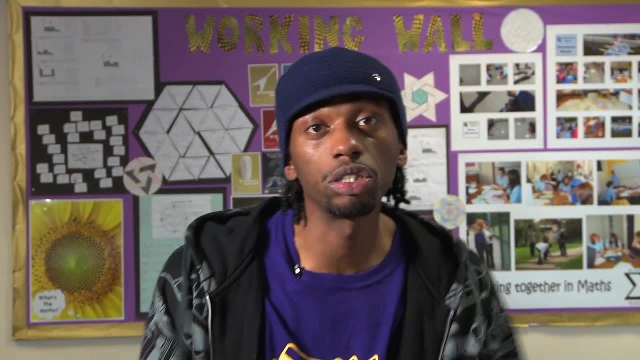 to go the other way, then we must divide. If you ever get a moment when you've got a problem, you can't decide From percentage to decimal. you just divide A fraction's a whole number over another. Just do the division to get the decimal number. A decimal's the 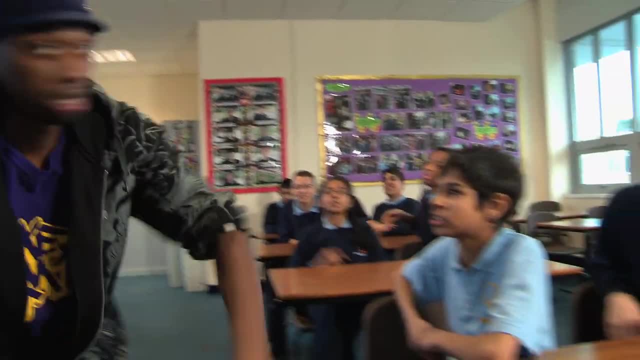 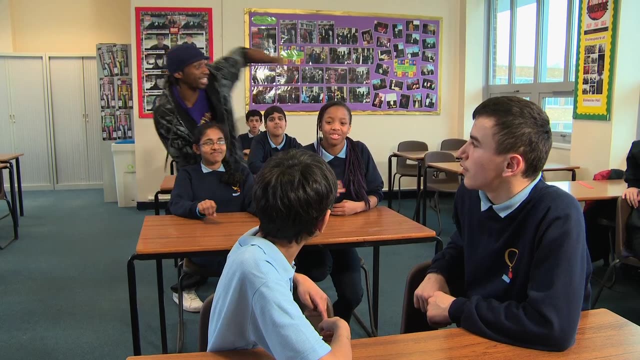 one with the point to remember, and if out of a hundred, a percentage is better. So all we're doing is assessing our proportions. like one, half and two quarters are equally important, and three over five is like six over ten, which is also point six, or even 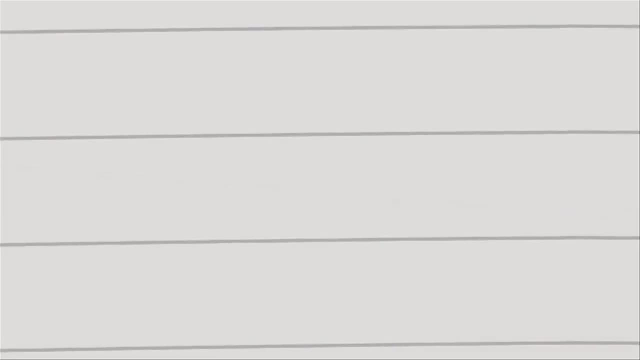 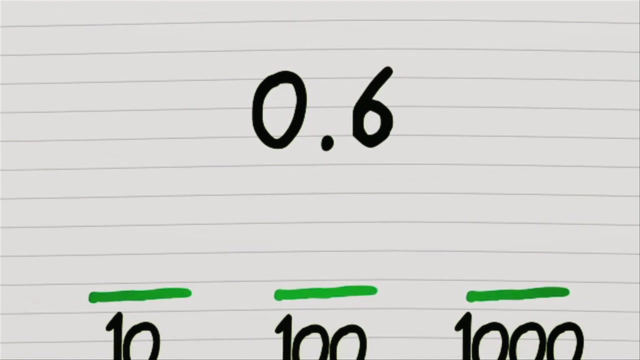 sixty percent. Now, to go from the decimal to the decimal, you just divide For percentage. decimals to the fractions. put the number over tens, hundreds, or thousands, Say. for instance, we took point six, ignore the decimal and leave the number. that's it. and if you're, 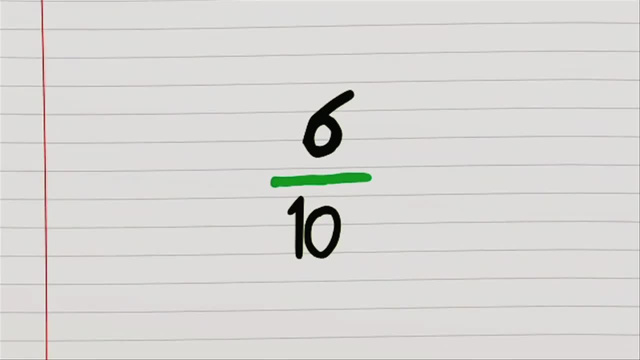 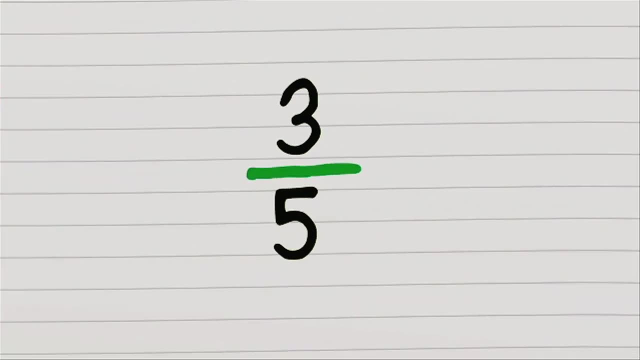 only left with one number. at the end, you're going to have to then divide the number by ten. The top and bottom may be divisible by the same things alike. Here we used two to finish up with three fifths. Now let's tackle zero. point six one. Ignore the decimal to. 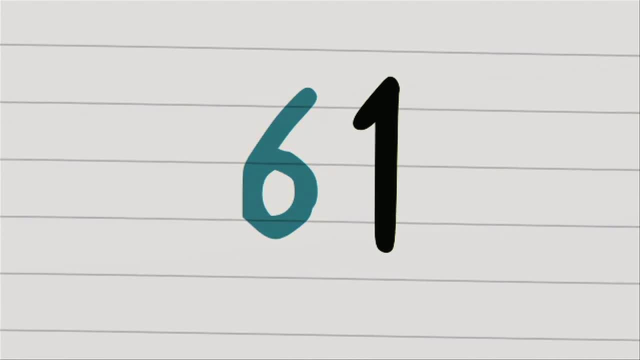 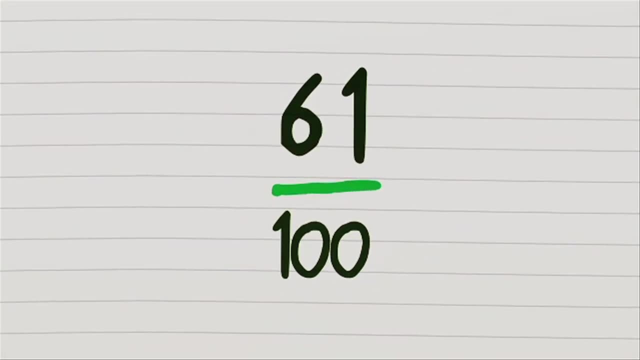 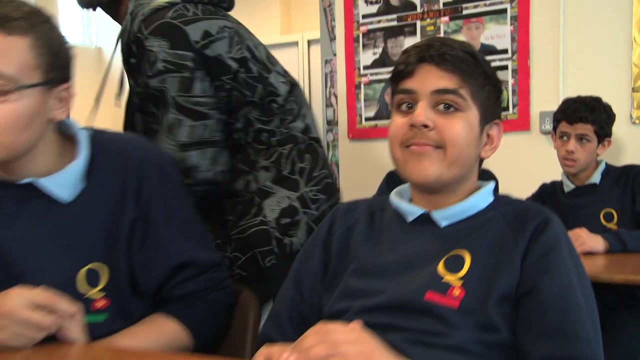 leave sixty-one To the right of the decimal. we had two numbers, so now we're going to put them over a hundred and one covered. his name as a fraction is sixty-one hundredths, with no numbers that can go into both. it won't cancel down and that's the end of the road. 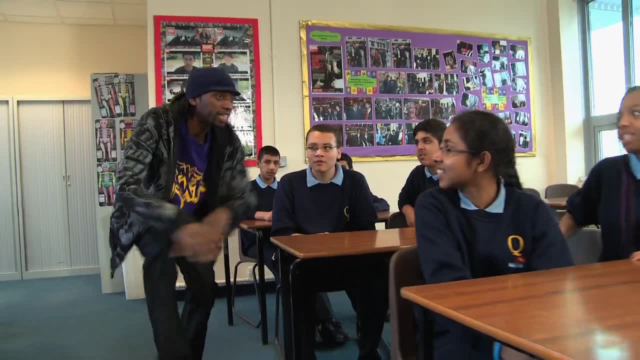 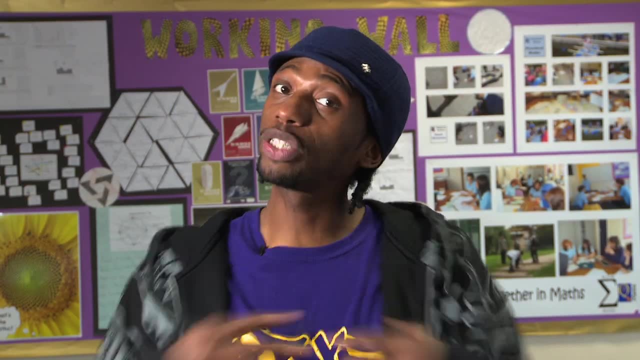 A fraction's a whole number over another. just do the division to get the decimal number. a decimal's the one with the point to remember, and if out of a hundred it's sixty-two. so all we're doing is assessing our proportions. like one half and two quarters are equally. 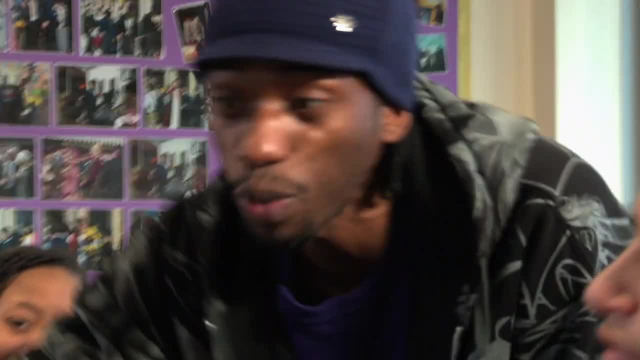 important, and three over five is like six over ten, which is also point six, or even sixty percent.